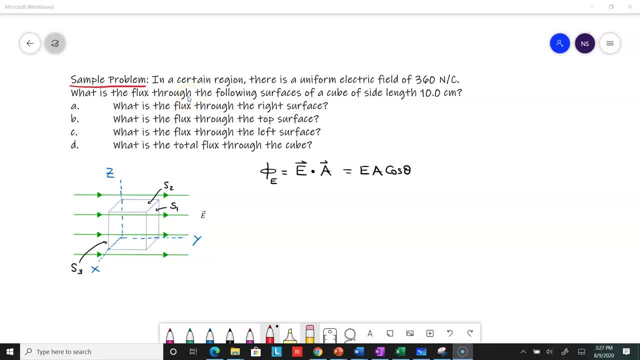 So here is the sample problem. It gives you a uniform electric field of 360 newtons per coulomb, And if I take my x, y, z axis the way I have shown here, that means the electric field right that is given as 360, here it is black: 360 newtons per coulomb in the positive j. 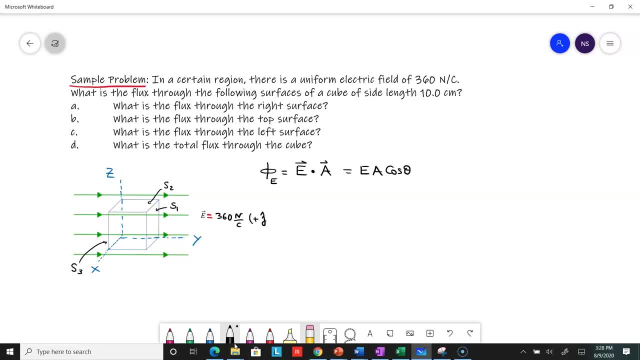 direction: right, It is in the positive j direction along the y axis, And you are asked to calculate the electric flux through the right surface, the top surface, and then the left surface and finally the total flux through the whole cube. Okay, And the length of the cube is also given to us. That is 10 centimeters, So I will. 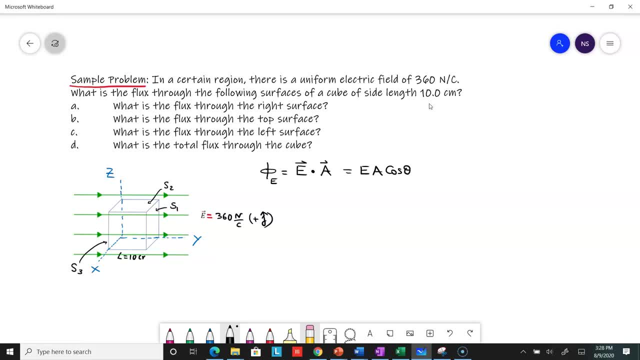 call it L. L is 10 centimeters Or I can convert that to meters, 0.1 meters. Okay, So in any of these problems where you have clean surfaces in an external electric field, a uniform electric field, you can just use the formula E dot A or E times A. 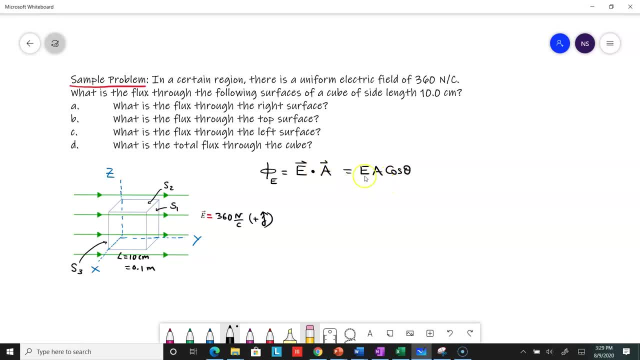 times cosine theta, And you can either use E A cosine theta or, if you prefer, you can write it in your calculator notation and take the dot product right. So however you prefer. So let us start with part A. What is the flux through the right surface? 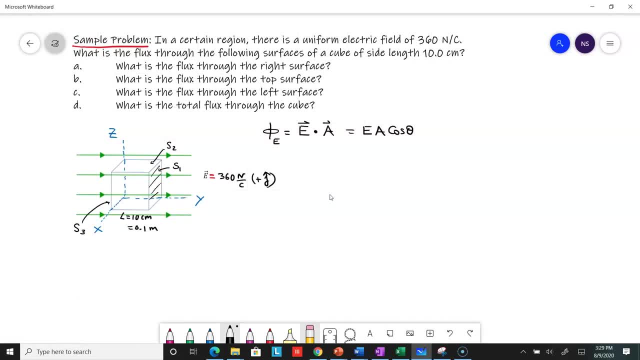 So the right surface is this one here. right, That is the right surface, S1.. And the area vector or the normal vector is the outward drawn normal. So that is the normal vector, which is also the direction of the area vector. So that is the area vector there. A. 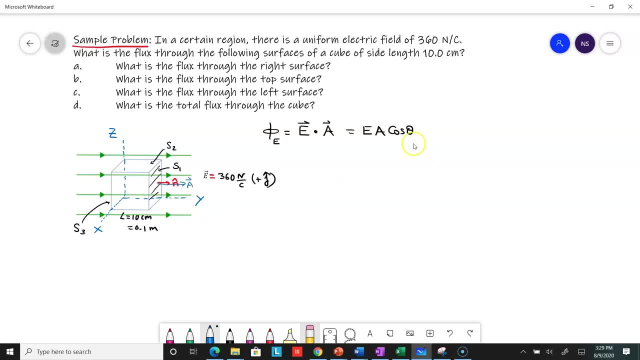 So let me first use the E? A cosine theta to calculate it. So flux phi E through the right surface- that means through S1, is equal to E A cosine theta. So it is E times A times cosine of the angle. 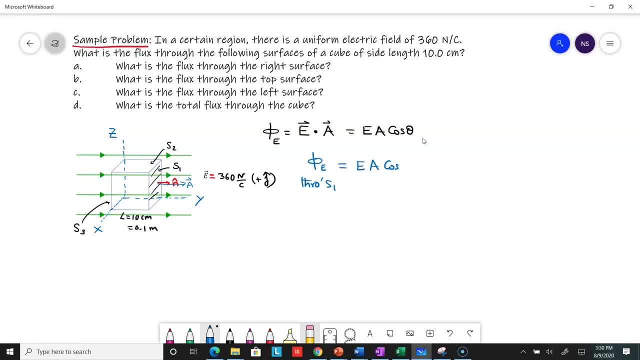 And the angle between the electric field. electric field is to the right and the area vector is to the right. So theta is zero here, cosine zero, So that is just E times A. So you just substitute your numbers: 360 newtons per coulomb, and the area is L squared or 0.1 meter squared. So 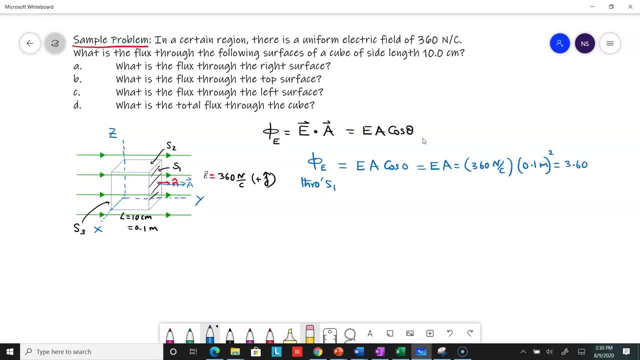 that will give you 3.6 Newton, So that is a positive flux. field lines are leaving the surface And similarly I could calculate the flux through the top surface. So if I look for the flux through the top surface, 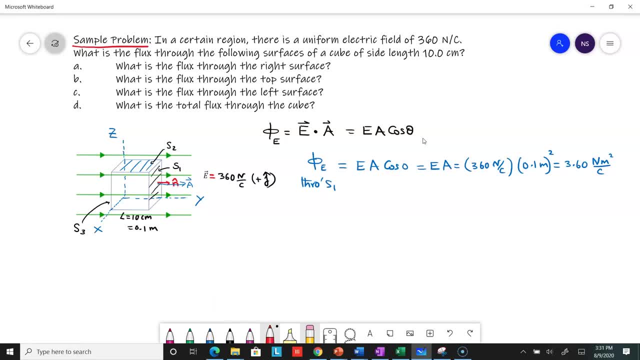 I have, my normal vector will be the outward drawn normal. So that is that way And you can probably right away say that. you know, the area vector is perpendicular to the electric field vector, right? So the electric field there is to the right. 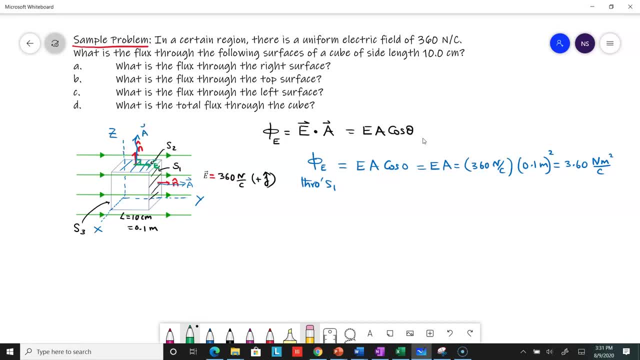 So that is 90 degrees. So there is no flux. or you can formally write it down. Now you can say: flux through S2 is E A cosine theta, So E times A times cosine theta, which is 90 degrees. So 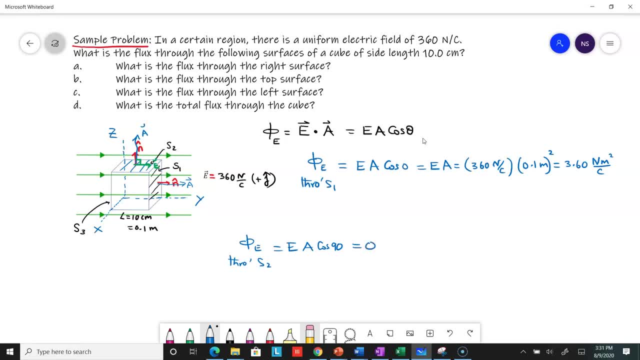 cosine 90 is 0. So this is just 0.. Right, Okay, that's my part B. so this was part B, this is part A, and I can also do the same for this surface. now right for S3, which is the left surface and the normal vector, for that is the. 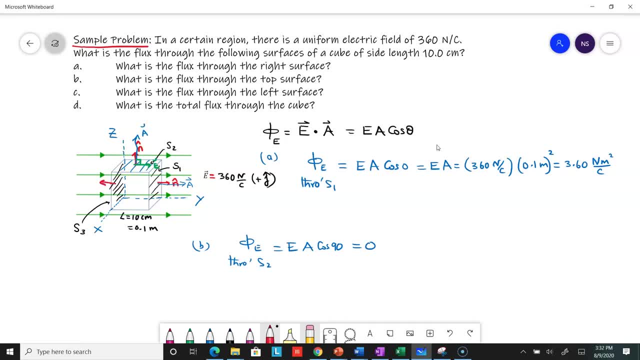 outward drawn normal. so that's this vector here, that's the normal vector which is also the direction of the area vector right. so area vector here is opposite to the electric field vector, or in other words the angle at theta is 180 degrees right. so you can go ahead and you can. 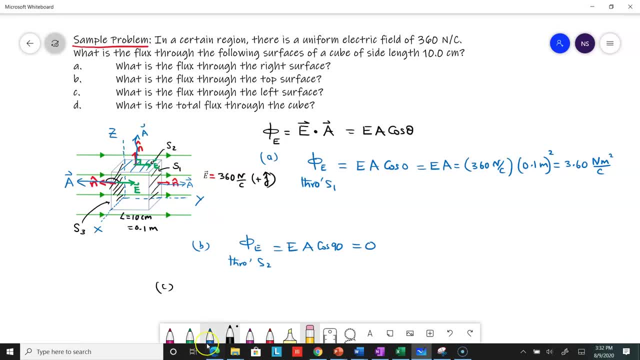 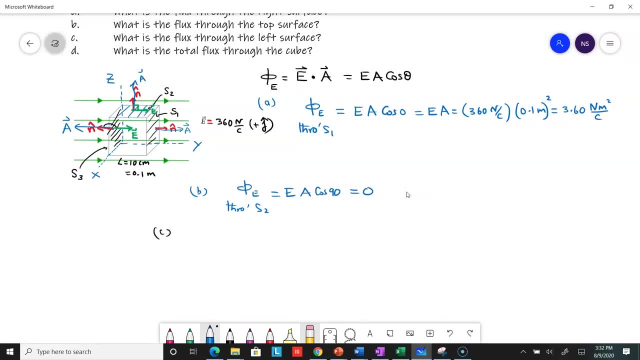 you can say part C is- let me make some space- part C is phi. E is equal to right Ea cosine theta, so it's Ea cosine 180 degrees, and these are the magnitudes. so so if you substitute everything you know, this is minus 1, that's your 360. 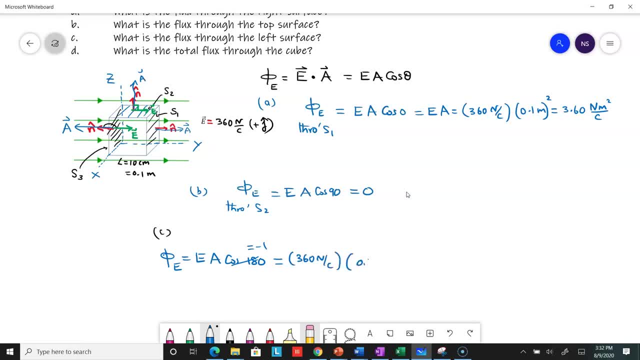 newtons per coulomb times 0.1 meter squared times cosine, 180 is minus 1, so you get the exact same value as 3.6, but it's negative. now, newtons meter squared per coulomb- okay. 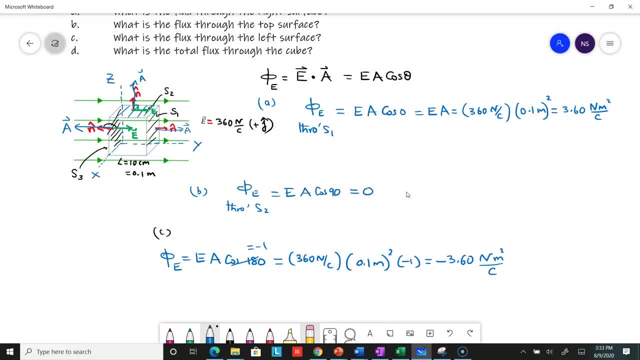 so. so once we have this, it's probably clear to say that. to go to part D, we could just see that the only non-zero flux is going to come from the right face, right face and the left face. we showed flux through the top face is zero. same reason, flux through the bottom face would be zero. 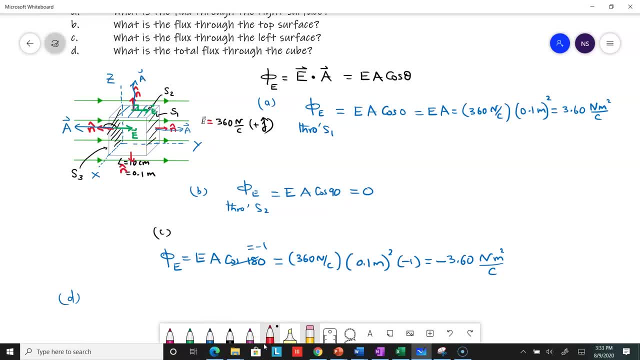 as well, because of flux through the top face is zero. so we can just start with the top and then we can start with the bottom face, because we can start with the top and then we can start with. the normal vector will be pointing downwards right and the electric field is perpendicular again. so 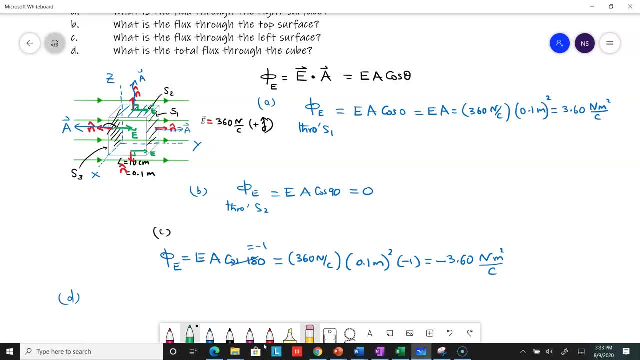 or you can say electric field vectors just skim along the surface. so no flux through that. and same reason, no flux through the front surface or the back surface as well. so we can say the total flux or the net flux right, a net flux through the cube right. 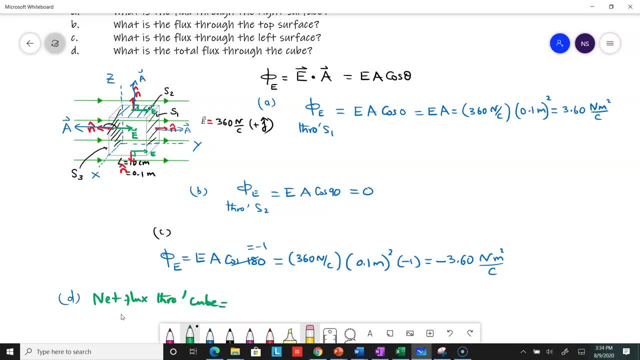 is just sum of all the fluxes, so that is a 3.6 plus a negative 3.6. right flux through all the surfaces added together will just give you a nice zero right. so this is another way to convince ourselves. since the electric field is constant, every field line. 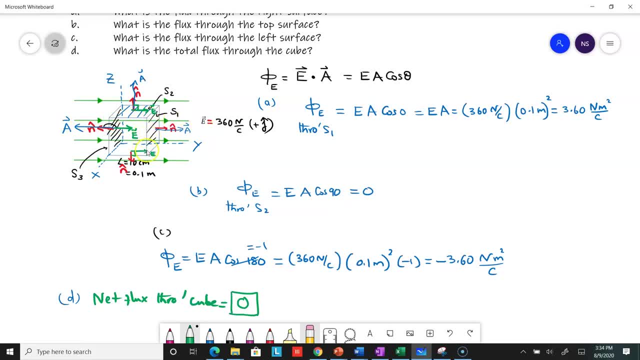 that's entering the surface is also leaving the surface. so it makes sense that the net number of field lines that leave the surface, which is the meaning of the net flux, that is zero. okay, so this is all you need to do, but in case you were trying to do this with, 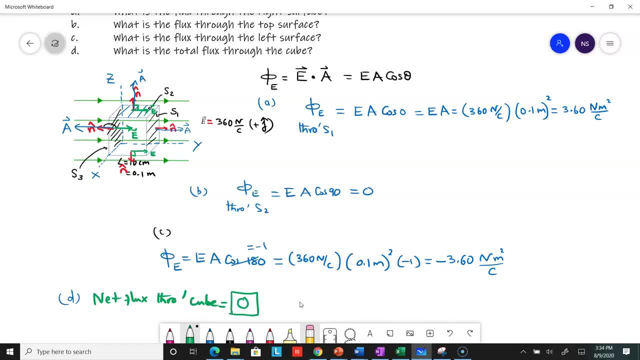 your calc 3 notation. that's totally okay as well. so for example, in part a, if you, if you rather wanted to set up a dot product, you could have certainly done. i'll say r? i you could have done phi e s, e, dot a. so the electric field has got no x component, it's got 360. 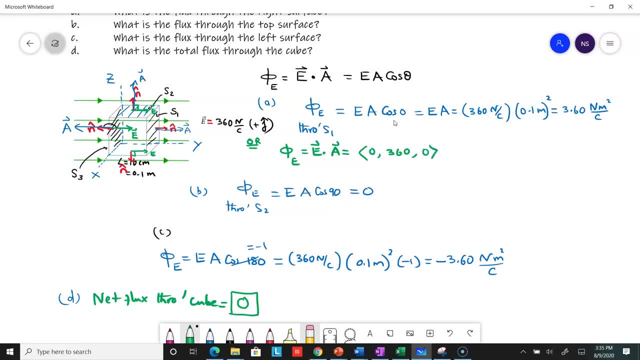 newton's per coulomb in the y direction, nothing in the x right. so newton's per coulomb are dotted with the area vector. for s1 the area vector is also in the y direction. so 0 comma, 0.1 meters. 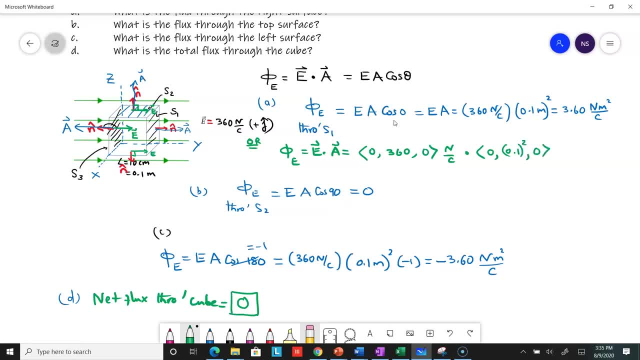 squared right: comma 0.1 meters. squared, so 0 comma 0.1 meters. squared right: 0 square meters. and that will give you, when you do the dot product, it will give you exactly the same thing. you see, the same way. if you were doing it here, you could certainly, you know. 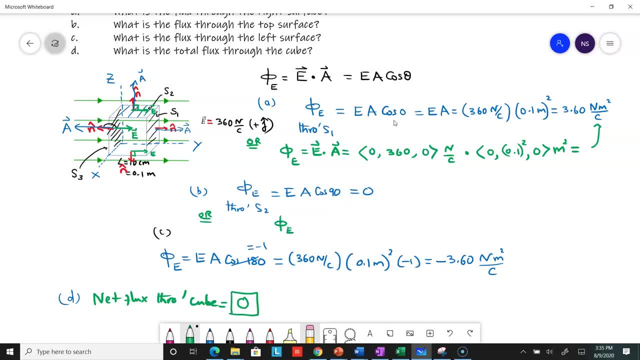 this is the dot product. so you can say phi e through s2 is e, dot a and your vector e is 0 comma, 360 comma, zero newton's per coulomb dotted with the area vector. and the area vector for the top one is along the z axis, so it is zero comma, zero comma 0.1 squared. 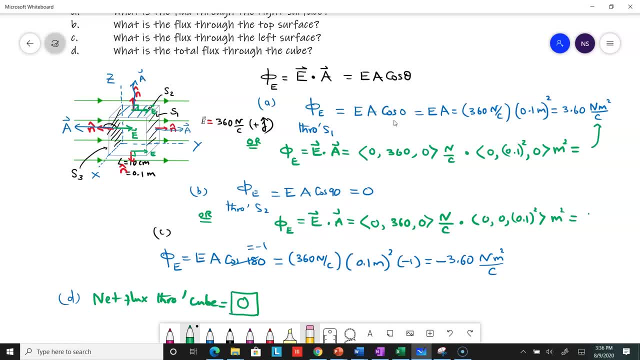 square meters and when you see, the dot product will be zero. you see, and you could have done the same thing over here. it's more of the same. uh phi, e is e, dot a. so here your e is the same thing: 0, 360 comma, zero newtons per coulomb, dotted with the area vector that points to the left. 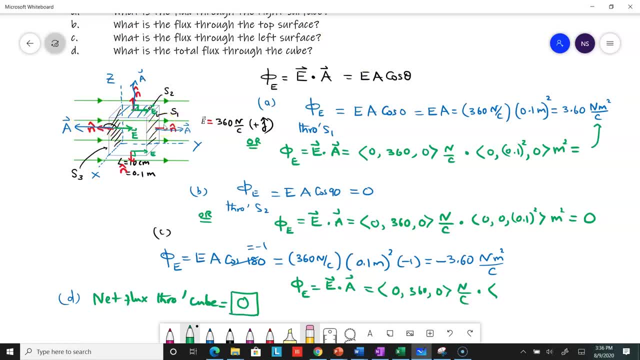 that's in the negative y direction. so you would have zero negative 0.1 squared eight comma zero square meters, and that will give you the exact same thing that you have, and you can end by calculating the total flux through the cube to be zero. So in general, I would just say: watch the. 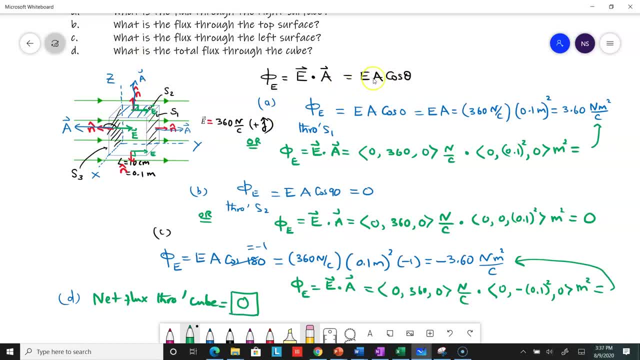 problem. in some problems, if the magnitudes of e and a are given and you can easily figure out the angle, this may be the quickest way to do the problem. but in some cases, if the e is given in the ij notation, perhaps it's easier to do the dot product instead of trying to figure out the 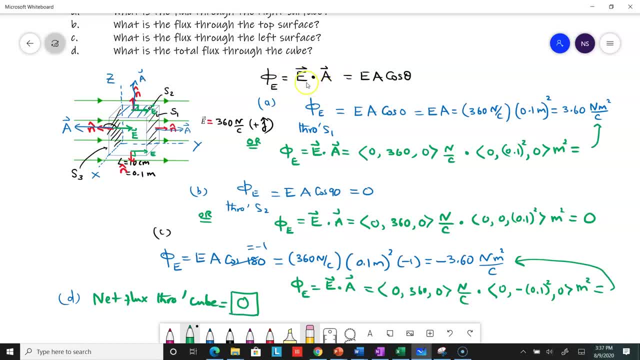 angles between the area vector in the electric field. Thank you for watching.